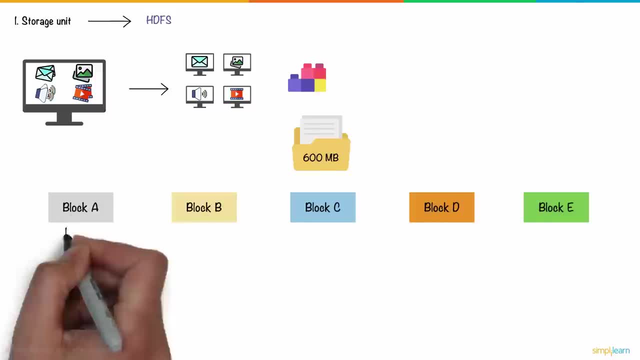 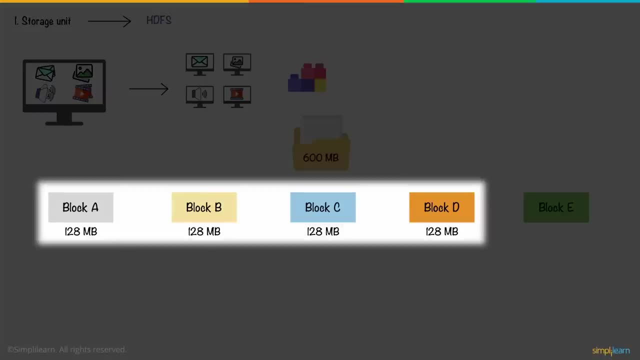 that are then stored on several data nodes in the cluster. 128 megabytes is the default size of each block. Hence 600 megabytes will be split into four blocks- A, B, C and D- of 128 megabytes each. 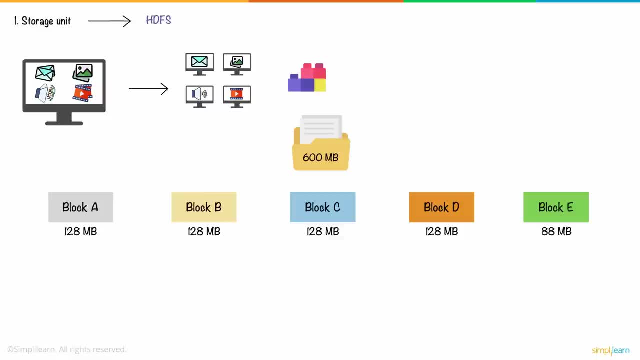 and the remaining 88 megabytes in the last block E. So now you might be wondering what if one data node crashes? Do we lose that specific piece of data? Well, no, That's the beauty of HDFS. HDFS makes. 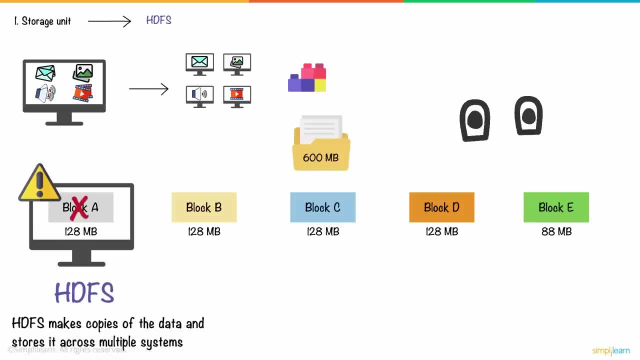 copies of the data and stores it across multiple systems. For example, when block A is created, it is replicated with a replication factor of 3 and stored on different data nodes. This is termed the replication method. By doing so, data is not lost at any cost, even if one data node crashes. 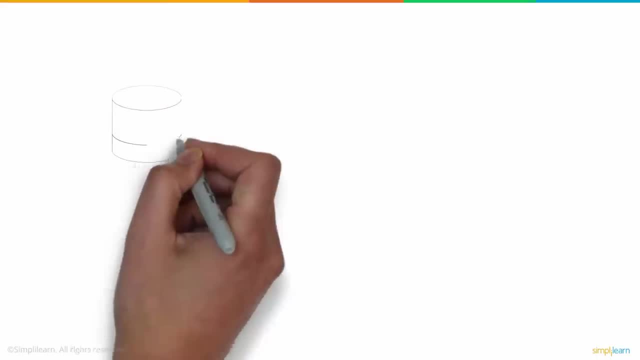 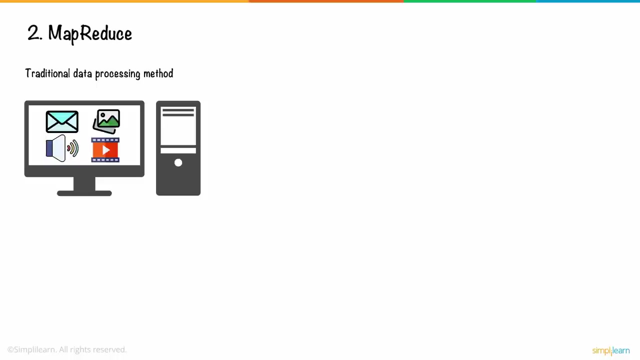 making HDFS fault-tolerant. After storing the data successfully, it needs to be processed. This is where the second component of Hadoop MapReduce comes into play. In the traditional data processing method, entire data would be processed on a single machine having a single processor. This consumed time and was 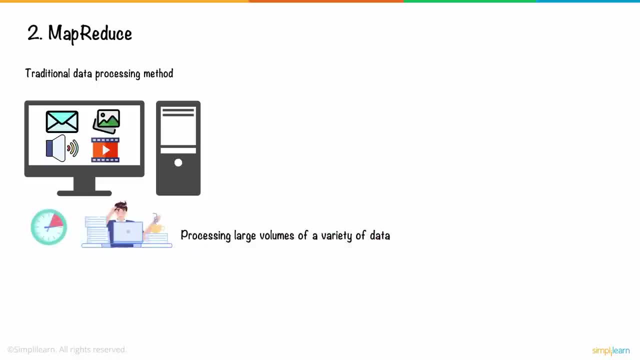 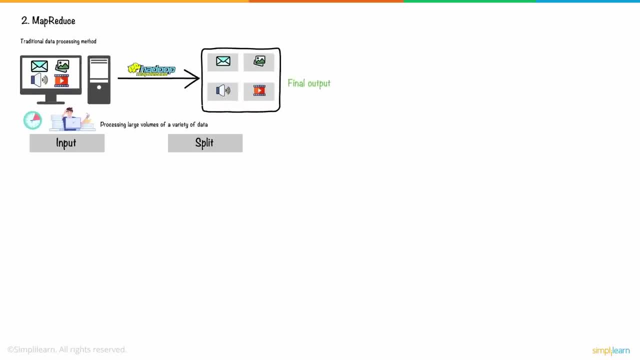 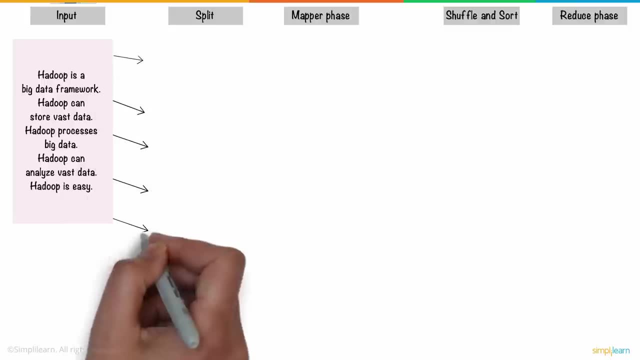 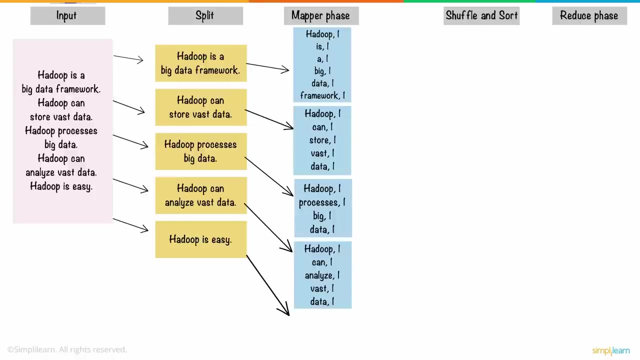 to give the final output. Let's try to count the number of occurrences of words. taking this example. First, the input is split into 5 separate parts based on full stops. The next step is the mapper phase, where the occurrence of each word is counted and allocated a number. After that, 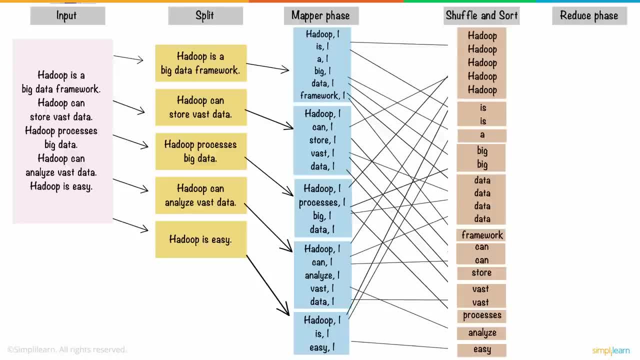 depending on the words, similar words are shuffled, sorted and grouped, following which, in the reducer phase, all the grouped words are given a count. Finally, the output is displayed by aggregating the results. All this is done by writing a simple program. 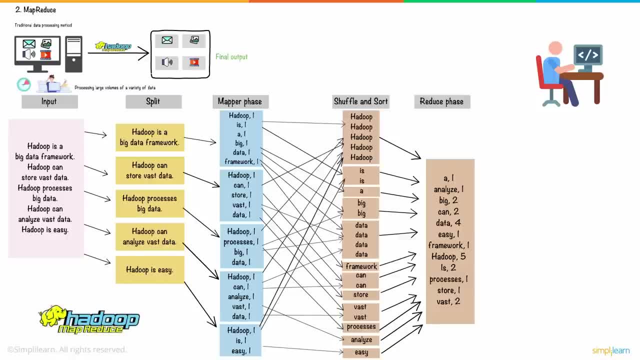 Similarly, MapReduce processes each part of big data individually and then sums the result at the end. This improves load balancing and saves a considerable amount of time. Now that we have our MapReduce job ready, it is time for us to run it on the Hadoop. 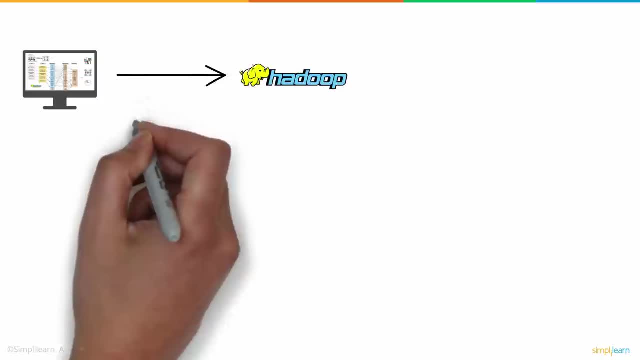 cluster. This is done with the help of a set of resources, such as RAM, network bandwidth and CPU. Multiple jobs are run on Hadoop simultaneously, and each of them needs some resources to complete the task successfully. To efficiently manage these resources, we have the third component of Hadoop, which 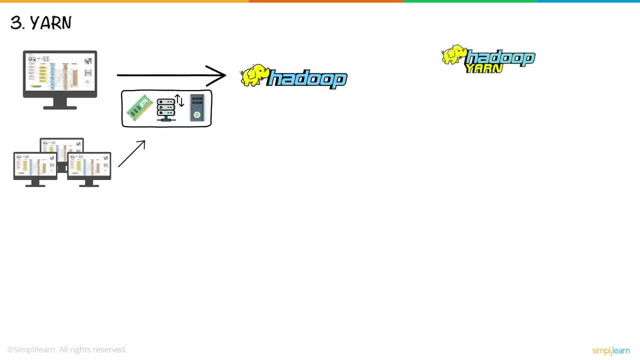 is YARN. Yet another resource negotiator, or YARN, consists of a resource manager, node manager, application master and containers. The resource manager assigns resources, Node managers handle the nodes and monitor the resource usage in the node. The containers hold a collection of physical resources. 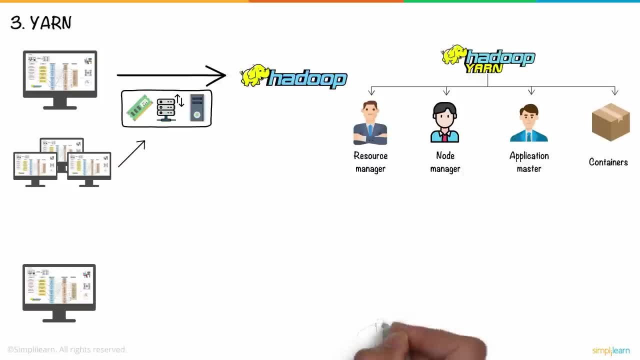 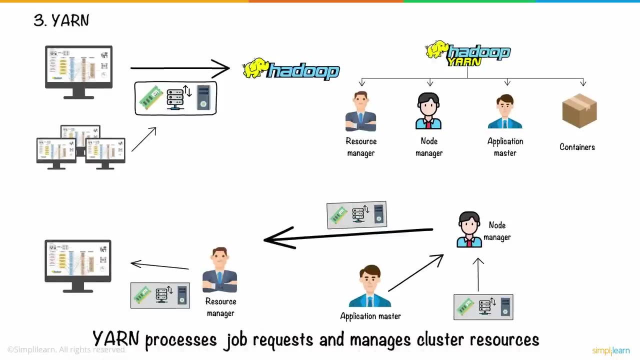 Suppose we want to process the MapReduce job we had created. First, the application master requests the container from the node manager. Once the node manager gets the resources, it sends them to the resource manager. This way YARN processes job requests and manages cluster resources in Hadoop. 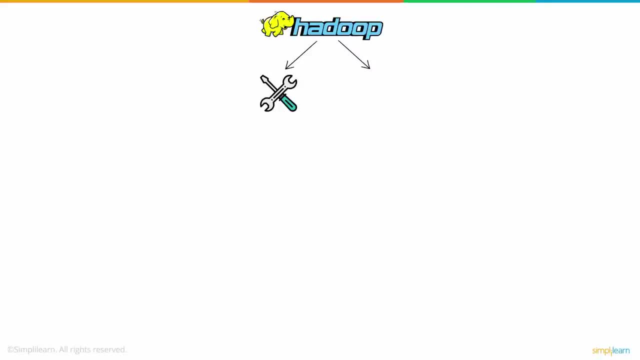 In addition to these components, Hadoop also has various big data tools and frameworks dedicated to managing, processing and analyzing data. The Hadoop ecosystem comprises several other components like Hive, Pig, Apache, Spark Flume and Scoop, to name a few. 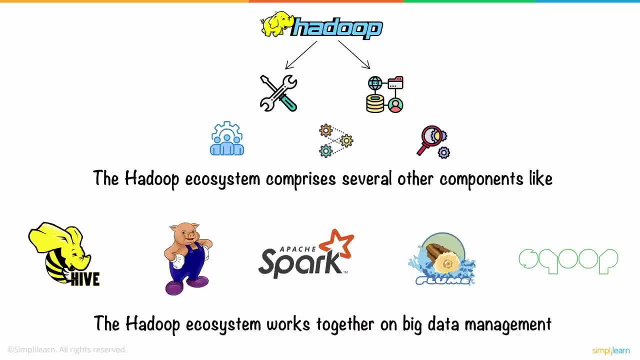 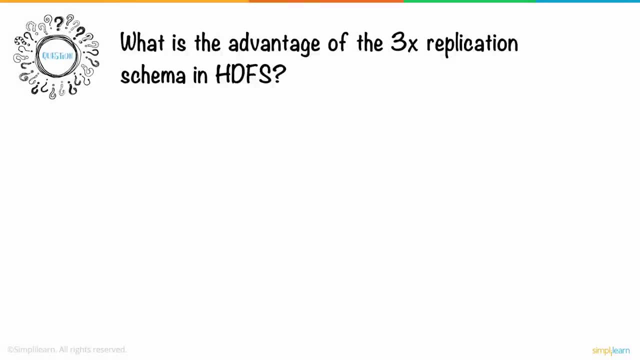 The Hadoop ecosystem works together on big data management, So here's a question for you: What is the advantage of the 3x replication schema in HDFS? A- Supports parallel processing. B- Faster data analysis. C- Ensures fault tolerance. D- Manages cluster resources. 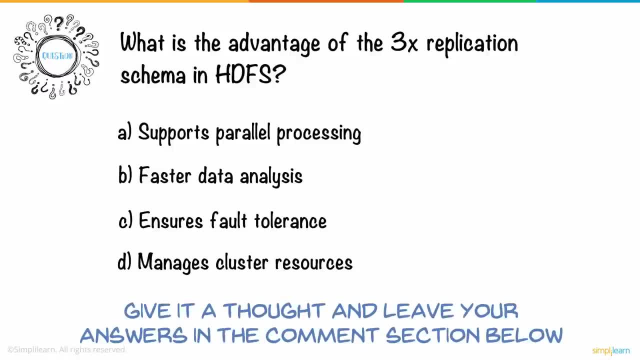 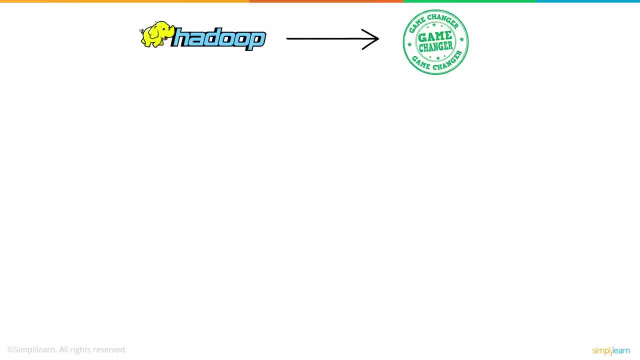 Give it a thought and leave your answers in the comment section below. Three lucky winners will receive Amazon gift vouchers. Hadoop has proved to be a game-changer for businesses from startups and big giants like Facebook, IBM, eBay and Amazon. 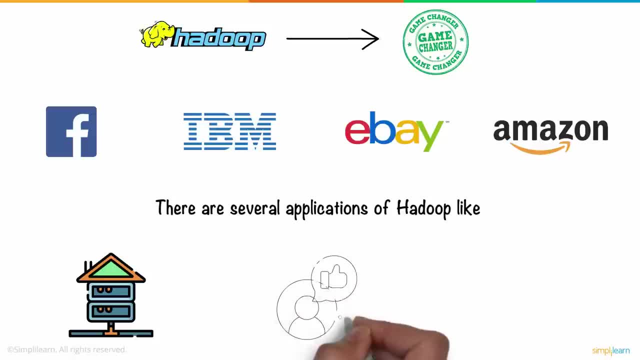 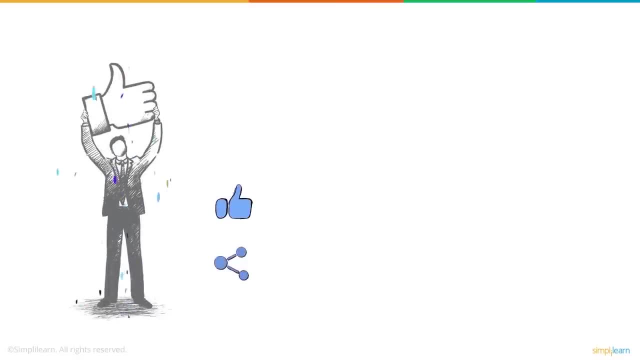 There are several applications of Hadoop, like data warehousing, recommendation systems, fraud detection and so on. We hope you enjoyed this video. If you did, a thumbs-up would be really appreciated. Here's your reminder to subscribe to our channel and turn on notifications so you don't miss.